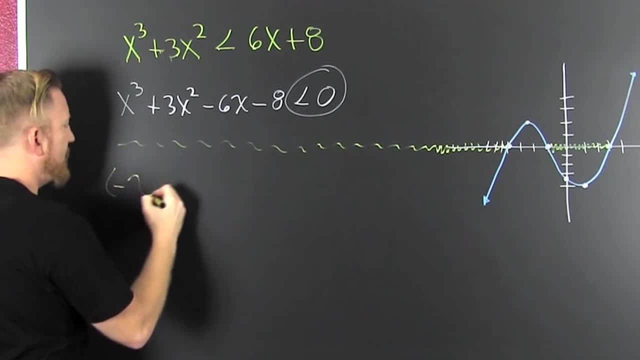 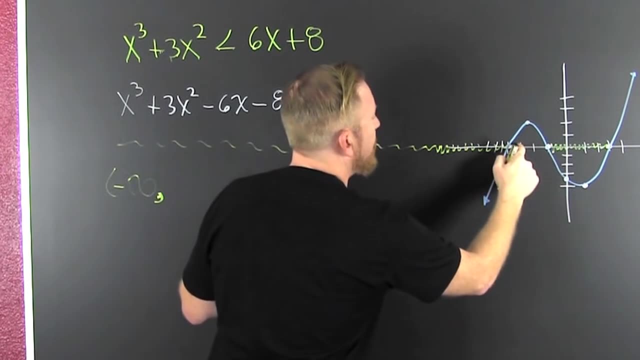 here. Where's the most leftist part? Oh, it's way over here at minus infinity. Okay, Uh-huh, And then to where? Looks like that's all the way: minus 1,, minus 2,, minus 3,, minus 4. So. 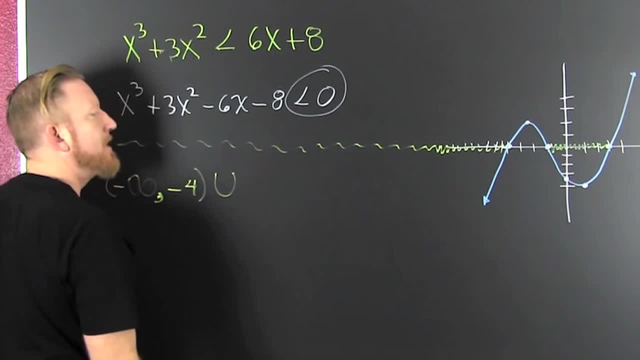 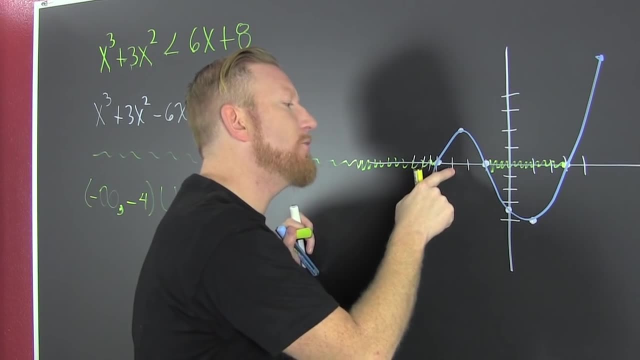 it's minus infinity to minus 4.. Sure, Then I'm going to go and I'm going to onion that up with what? This I'm looking for where it's below the line, What This blue one is, below that white one, when x is in between minus 1 and minus 2.. So I'm looking for where. 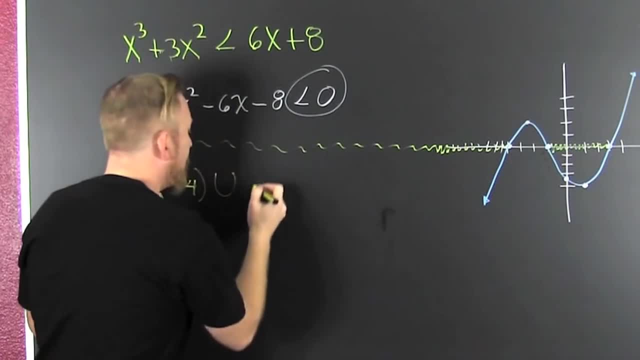 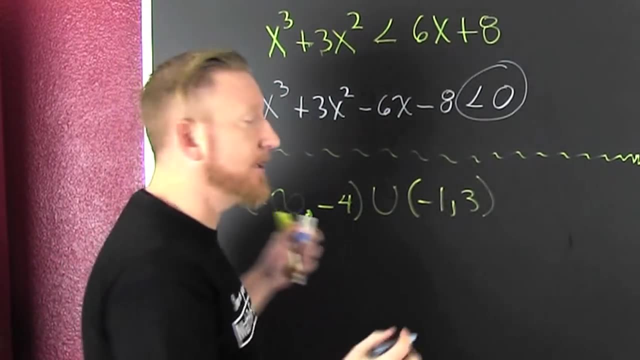 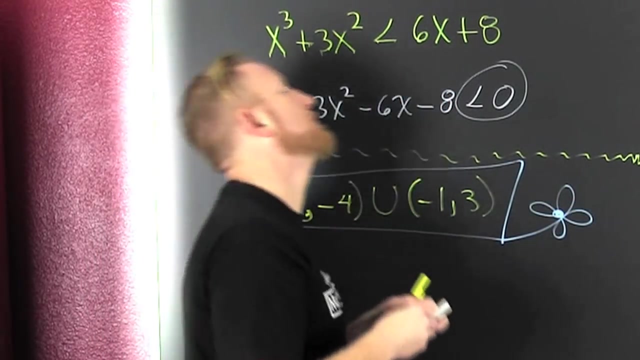 1, 0, 1, 2, 3.. Ah, So that's a minus 1,, 2, 3.. Onion that up. and then what? Boxing flower? Sub-zero. finishing Boxing flower. 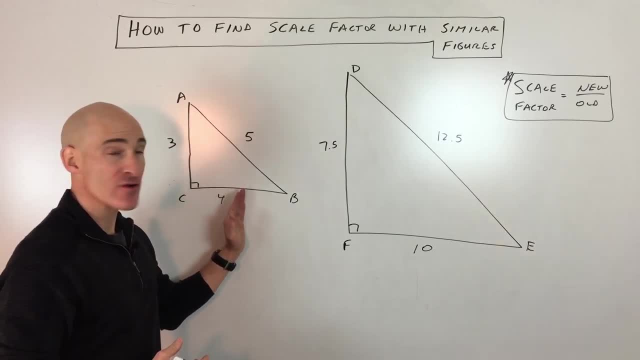 Well, you want to know whether you're finding the scale factor from this figure on the left to this figure on the right, or if you're going from the figure on the right to the figure on the left. So that's very important is the direction that you're scaling the figure And the formula. 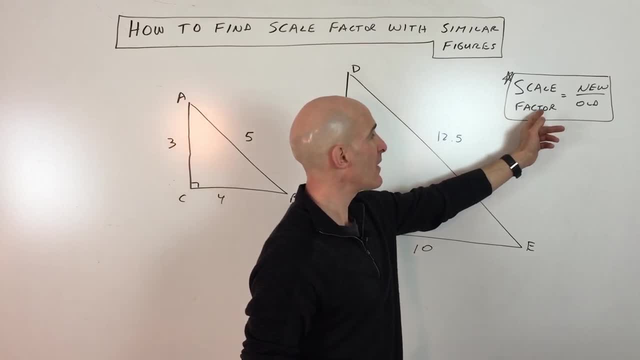 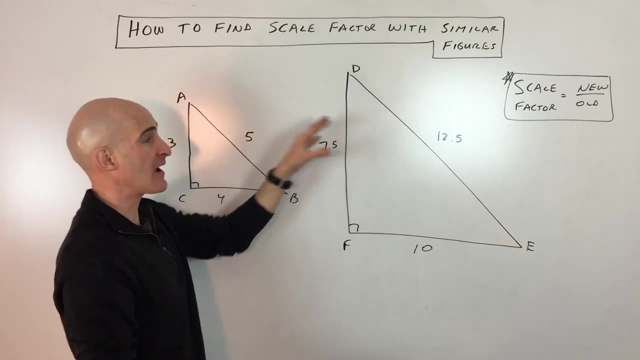 I like to remember. this is just a simple way of doing. it is just think about new divided by old. So if I'm going from this triangle to this triangle, this is my new triangle and I'm going to divide by the old triangle. Now what you want to do if the figures are similar and they tell. 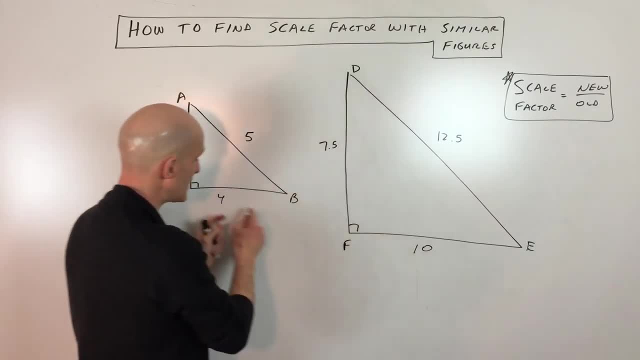 you that in the problem you want to match up the corresponding size. So say, for example: if I'm comparing 4 and 10, I'm going from 4 to 10, what am I multiplying by to get from 4 to 10?? That's. 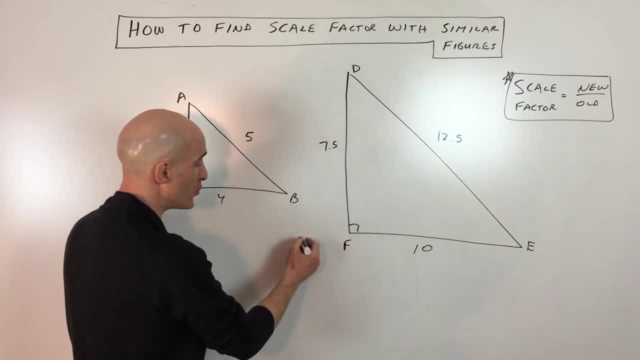 my scale factor. So the easiest way to do this would just be to take the new length, which is 10,, divided by the old length, which is 4, and you can see that's giving us a scale factor of 5 divided.